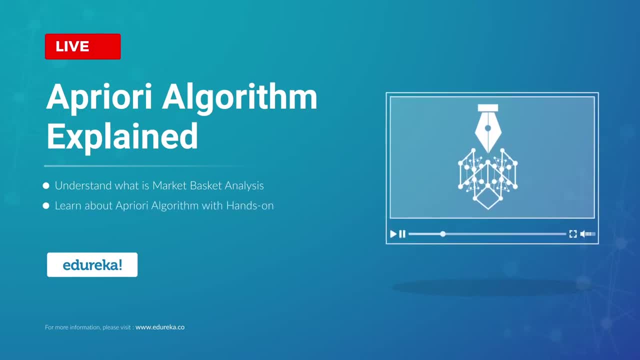 So good morning, good afternoon and good evening, guys, based on the time zones you all are coming from. So, guys, before we start with the session, can you all please give me a quick confirmation, if you all can see my screen and hear me loud and clear as well? 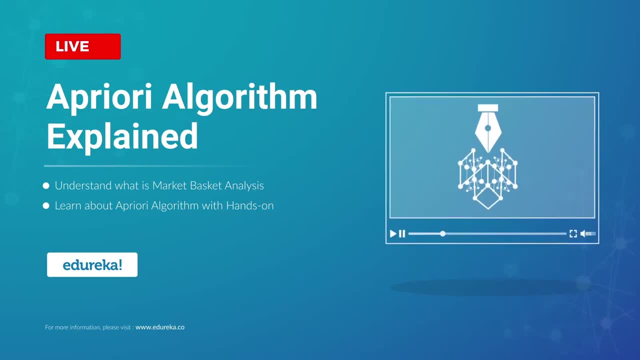 Perfect. Thank you so much for the confirmation, everyone. So my name is Neeraj Kheria and I have been working in this IT industry for more than 13 years now. So the main agenda for today's session we are going to discuss on the market basket. 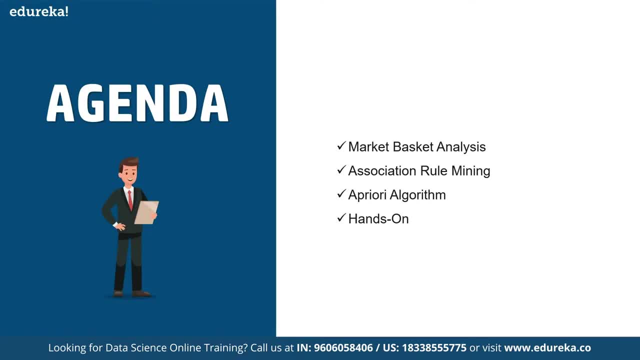 analysis here how the association rule mining works and how the Apriori algorithm works. A small question that we can start with is: has it ever happened that you are out to buy something and you end up buying a lot more than you have planned? So this normally happens. 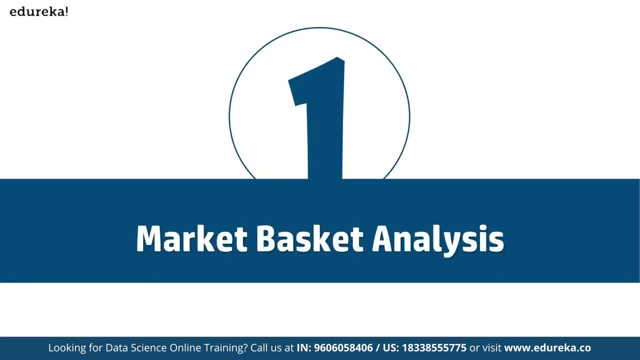 in the marketplace is correct. So it's a phenomenon called as the impulsive buying, and big retailers take advantage of machine learning and Apriori algorithm to make sure that we tend to buy more, and that's what we have defined as a market basket analysis. Now first. 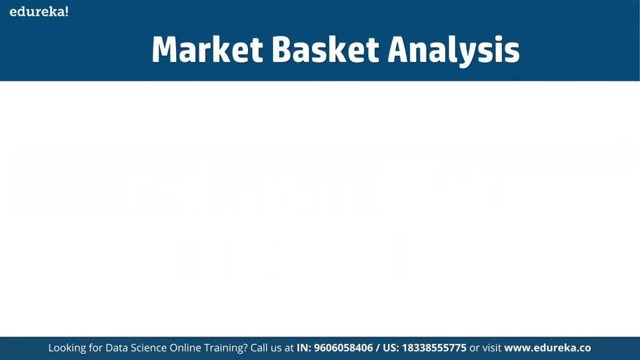 of all. let's discuss on that. So in today's world, the goal of any organization is to increase the revenue, And can this be done by pitching just one product at a time to the customer? The answer is clearly a no. Hence the organization began mining data related to frequently bought items. 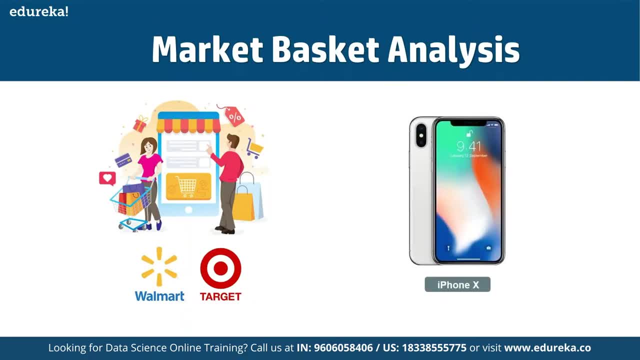 So market basket analysis is one of the key techniques used by large retailers to uncover associations between items. So they tend to find out the associations between different items and products that can be sold together, Which gives assisting in right product placement. Typically it figures out what products are being 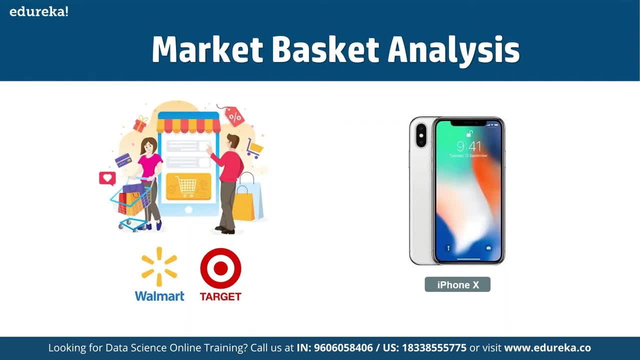 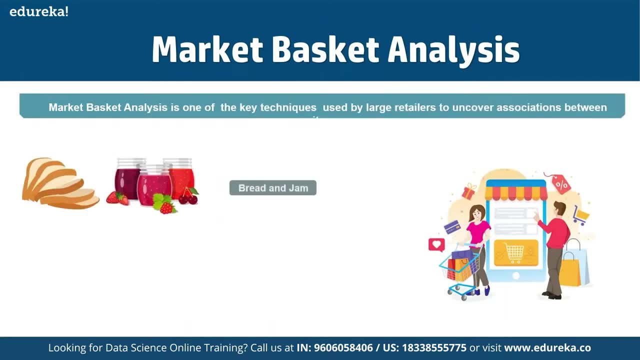 bought together and organizations can place products in a similar manner. Now let's understand this better with an example. Let's say we have people like people who buy bread usually buy butter too. So the marketing team at retail stores should target customers who buy bread and butter and provide them. 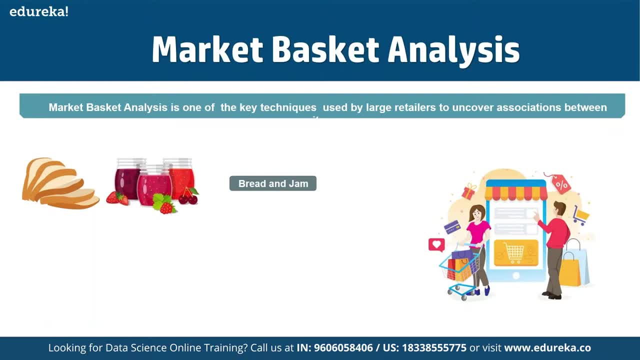 an offer to them So that they buy the third item, that we have eggs or any kind of jam as well, correct? so if a customer buys bread and the butter and see a discount or an offer on eggs, they will be encouraged to spend more and buy the eggs. so this is what market basket analysis is all about. so this is a small 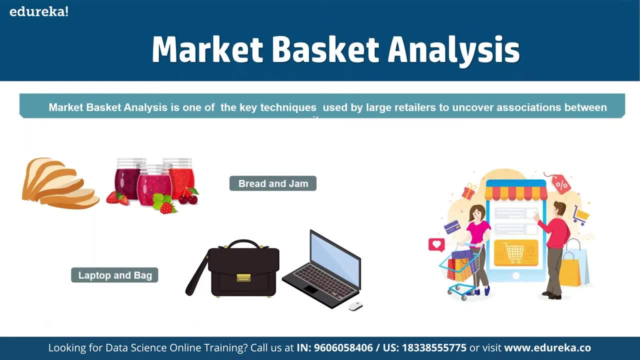 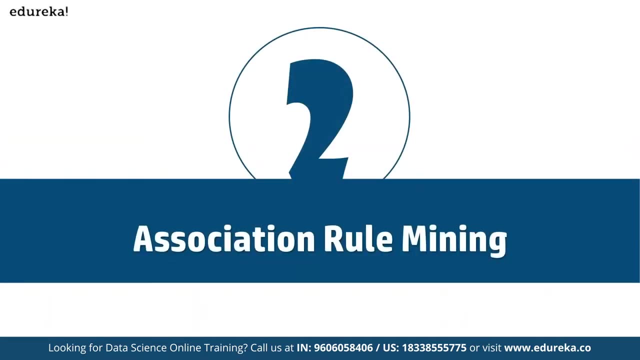 example, let's say, if we take thousand, ten thousand items data of our supermarkets to our data scientists, just imagine the number of insights we can get out of it. and that is why association rules mining is also important to understand. so if we talk about association rule mining, then 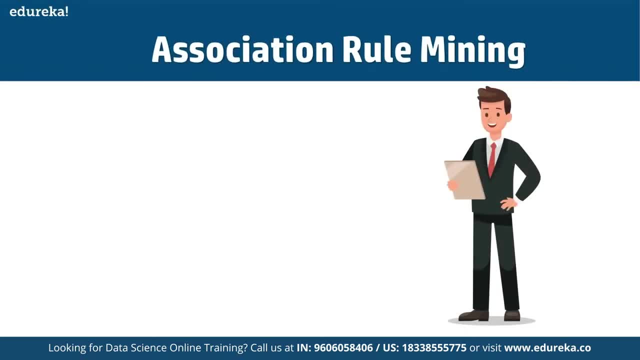 association rules can be thought of as an if then relationship. suppose we have an item a, so item a is bought by the customer and then the chances of an item b being picked by the customer to the same transaction id is found out. so here we have simple if and then relationship. so there are 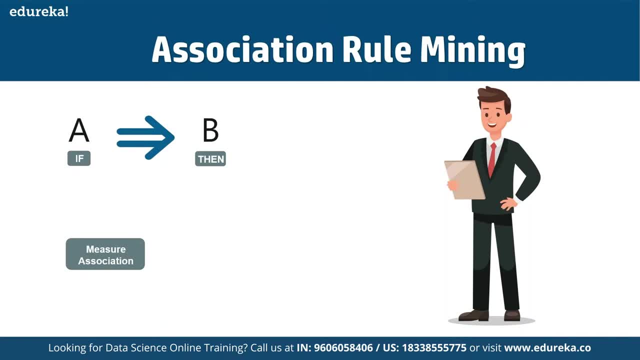 two elements of these different rules. first of all, we have the antecedent as an if so, this is basically an item or a group of items that are typically found in the item sets or data sets, and then we have the consequent. that is then so here we have then so then is basically used for. 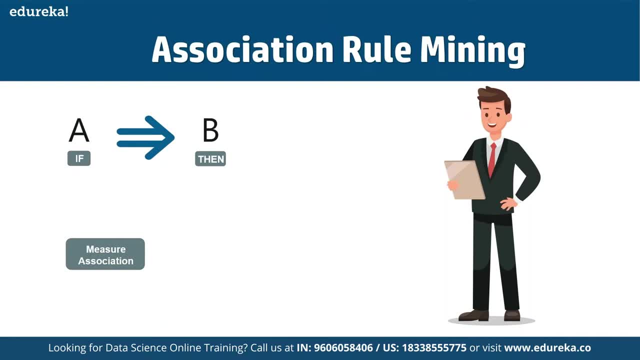 then it comes along as an item with an end event. that is then so then is basically used for then it comes along as an item with an end event, antecedent, or we can say a group of antecedents that we are seen and and this item we have discussed. 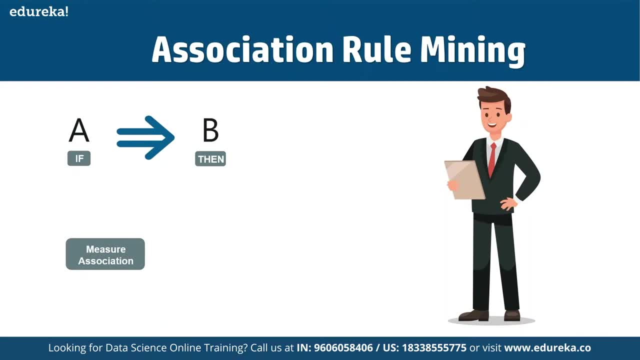 It is basically an item or group of items that we found in item sets of data sets. Now here comes a constraint. suppose we made a rule about an item use. We still have around 9999 items to consider for rulemaking, as we discussed. we have, we are going. 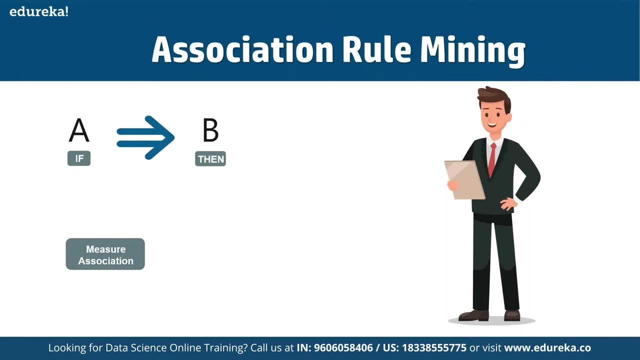 to make use of 10,000 items. So this is where apriori algorithm comes into play. So there, before we understand the apriori algorithm, let's understand the mean mathematics involved in here. So there are three ways to measure the association. 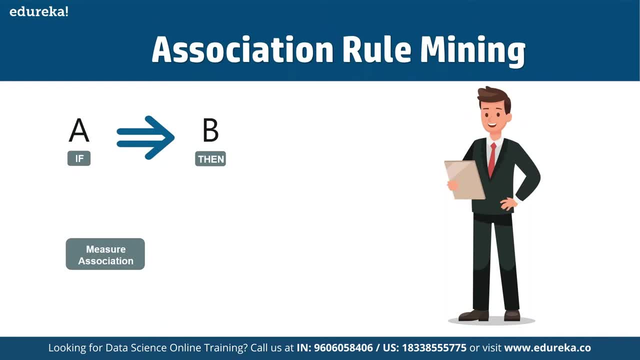 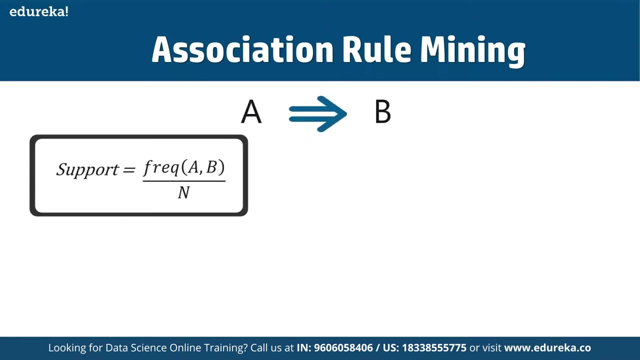 We have support, confidence and then we have lift. so, as you can measure the association here, We have support, confidence and lift. so support gives the fraction of transactions which contain items. A suppose, if you talk about support here, it is basically a frequent fraction of transactions. 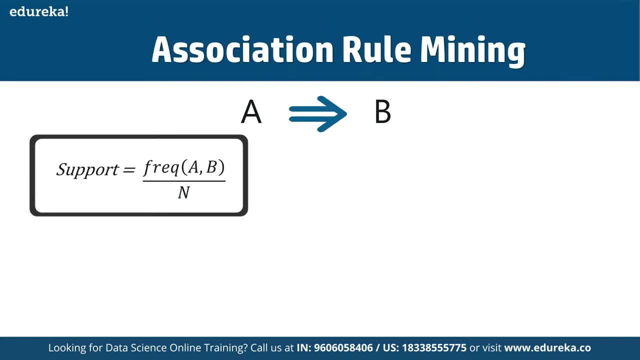 which contains item A and B. So basically, support tells us about the frequency for the organs that we can say frequently bought items or the combination of items bought frequently by using the support. So with this we can filter out the items that have a low frequency. then we have confidence. 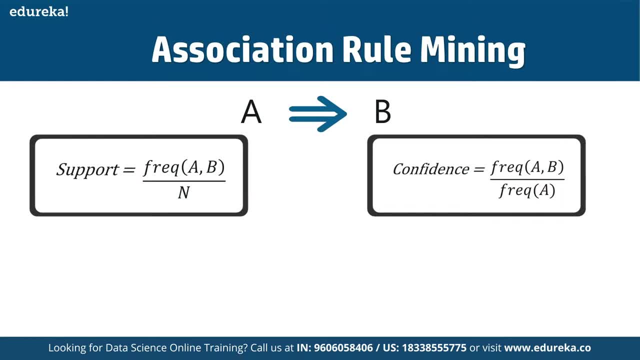 So it tells us how often the items A and B occur together, given the number of times a occurs. So typically, let's say, when we work with the apriori algorithm, we define different terms accordingly, but how exactly we have to decide the value. 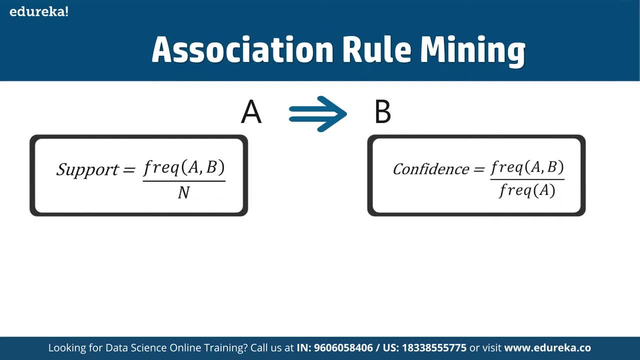 That's the main question And, to be honest, there is not a specific way to define these terms. Suppose we have assigned the support value as 2.. Now what is? What exactly this means is until and unless the item frequency is not 2.. 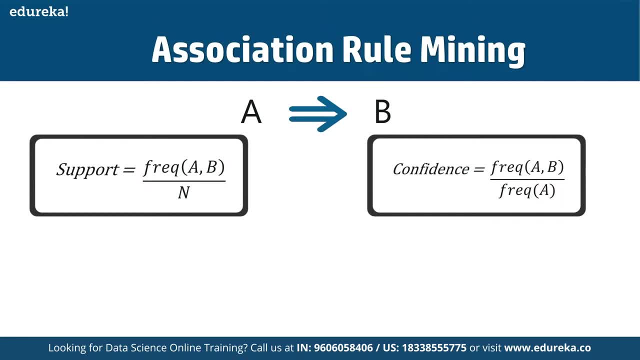 So here we define support as 2.. So until unless the items frequency is not 2%, we will not consider that item for the apriori algorithm. So this makes sense, as considering items that are bought less frequently is a waste of time because, let's say, if only 2% of users are, you are buying this item. 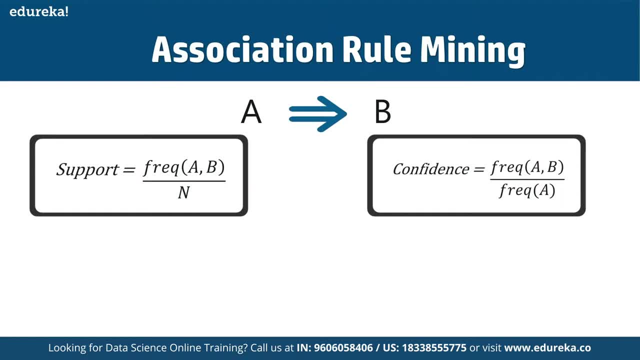 along with the item that they have bought, then obviously they will take it on use. Suppose that we cannot even consider is for the apriori algorithm that we are going to work on here. Now. suppose after filtering we still have around 5,000 items left. 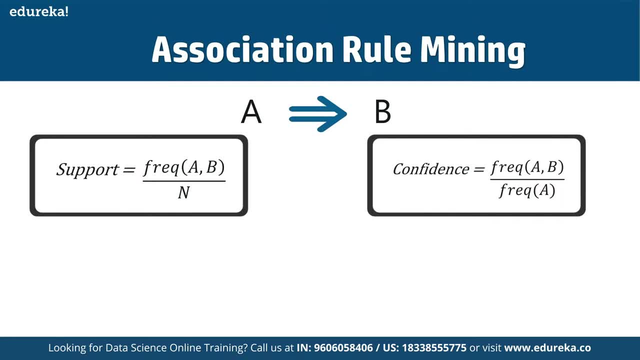 now, creating Association rules for them is a practically impossible task for anyone, and this is where the concept of lift comes into play. So, basically, lift indicates the strength of a rule over the random occurrence of A and B, and it basically tell us the strength of any given rule here. 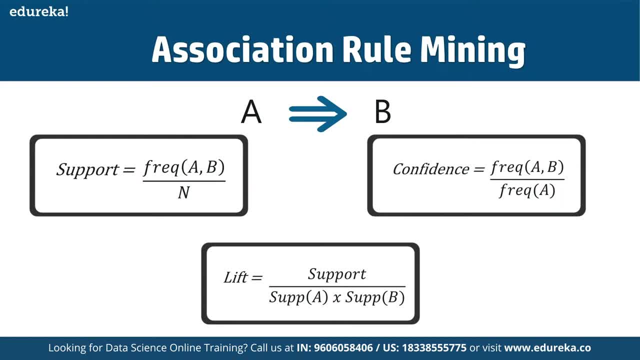 So for finding that out, we have to simply divide support with the by the support, by the support of A and then support of B. So focus on the denominator. It is the probability of the individual support values of A and B, and not together. So lift explains the strength of a rule. 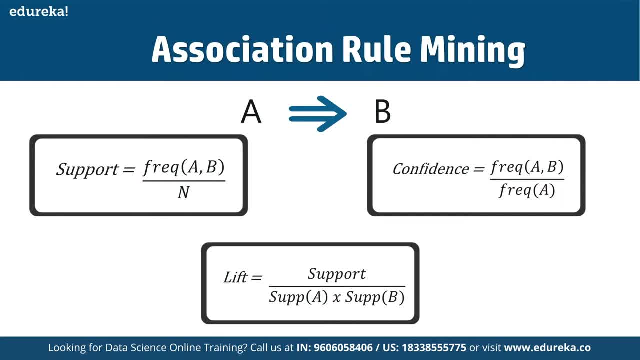 So more the lift, more is a strength. Let's say a as opposed to what we can say for a is to be. so if a, if, then relationship before. so if you talk about if, then relationship for a, B, then that lift value is for suppose. 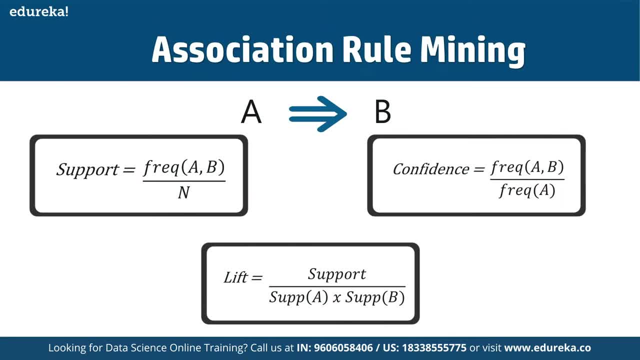 let's say, for this reason the lift value is for here. That means if you buy a, then the chance of buying B is four times if the lead value is four. or we can say it's four times if the value here is two, that it is two times. 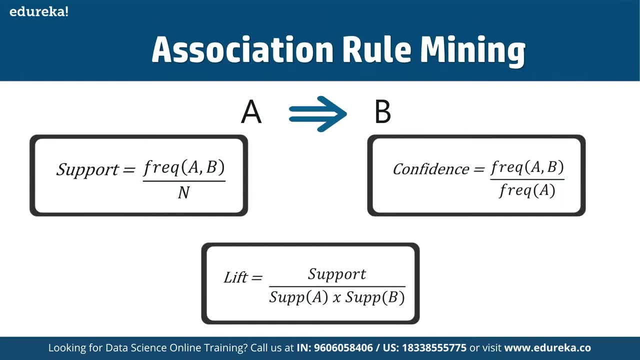 and so on, as a part of the lift values of fine. So let's get started with the a priori algorithm and now let's see how exactly it works. All right, So now let's discuss on the consign. This is what we discussed here. 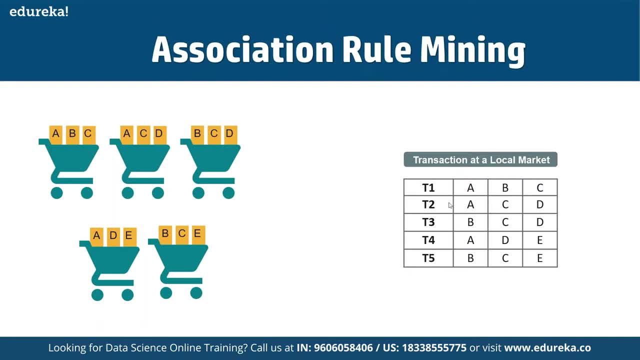 The transitions at local market. and here we have ABC for a in transition to we have a CD in transition. three: We have BCD in transition for we have ADE and then we have to transition five, We have a BCD. So let's say here: 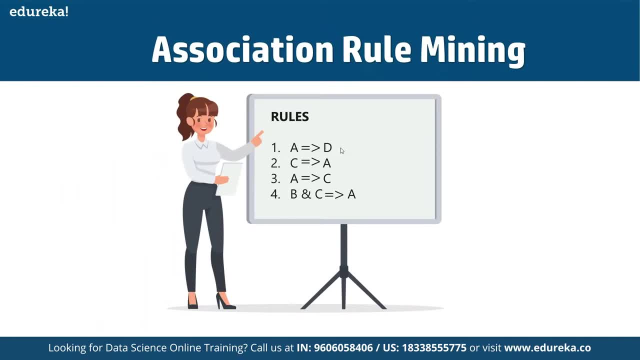 If you find out the entire rules here, then a. if a, then again they are going to purchase D. if they buy a seed, again they have the option of going for a. if they buy a, then they have the option of going for C, and if they buy B and C together, 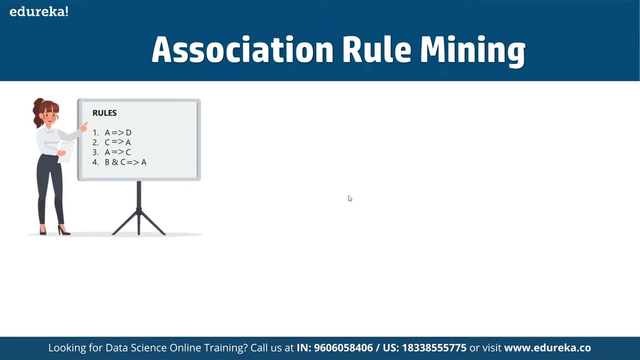 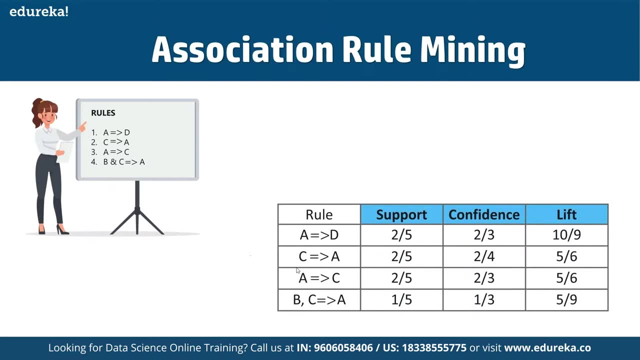 then they are going to buy by a as well, And then, same way, we can find out the support. So again for, if a is for those who are purchasing a, the probability of buying D, it is some in terms of support, It is 2 by 5 in terms of confidence. 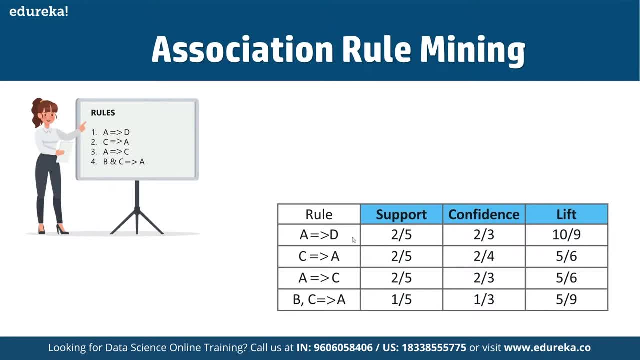 It is 2 by 3. in terms of lift, It is 10 upon. We ask for C again for a. that means what is, what is a possibility that those who have purchased C will be buying a. so you can find the support as 2 by 5 conference at 2 by 4 and lift us 5 by 6. same way. 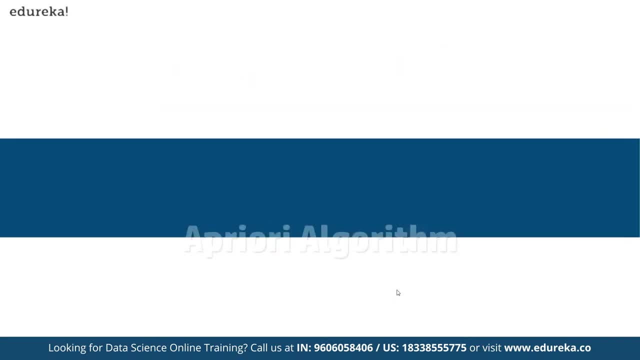 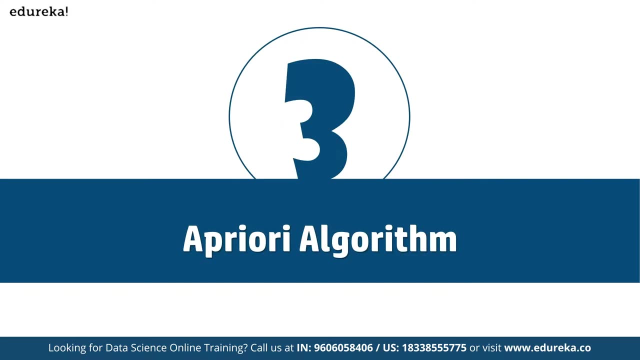 for C and same way for BC and a. so we can see how the probability is going to be distributed as we post, as we find out the possibility of one product to be bought over the other. All right, So now let's assume further on the a priori algorithm. 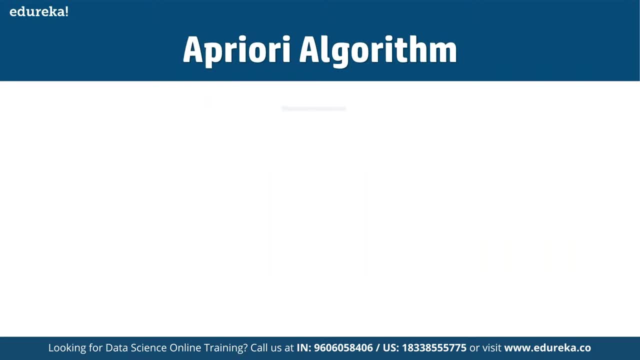 But so a priori algorithm uses frequent item data sets against item sets or data sets to generate the Association rules. So it is based on the concept that a subset of a frequent item set must also be frequent item set must be a frequent item set, and frequent item set is item set whose support value is greater. 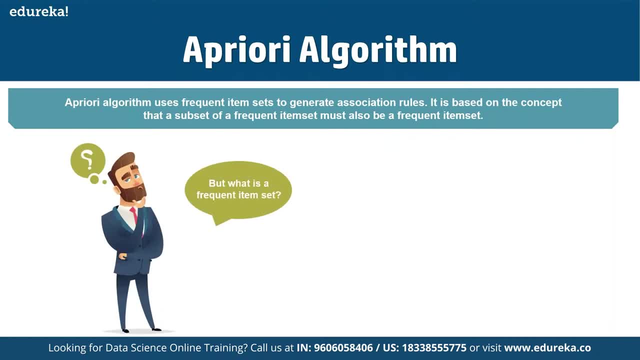 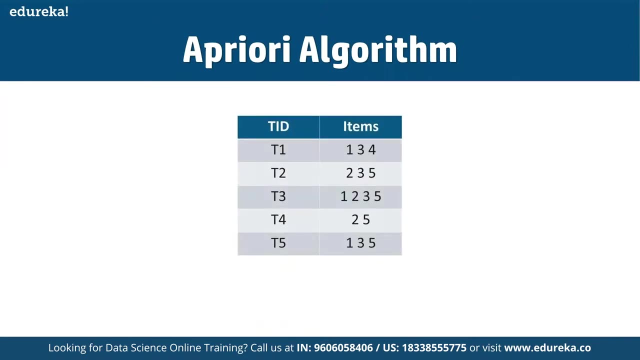 than a threshold value, that we have support. So let's say we have. now we're getting what exactly a frequent item set is. what we discussed as now is an item set whose support value is greater than a threshold value. All right, So now, if you talk about a simple example, now here we can. let's say, 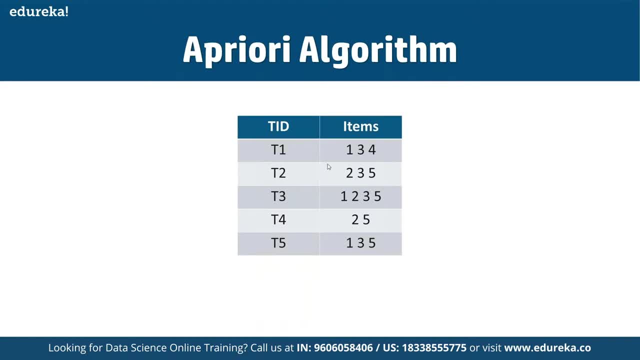 we have the following data of a store here. So we have the transition ID here, and then we have nine items. So here we have these. one are transition IDs and here we have the items. So in transaction one we have one, three, four, two. 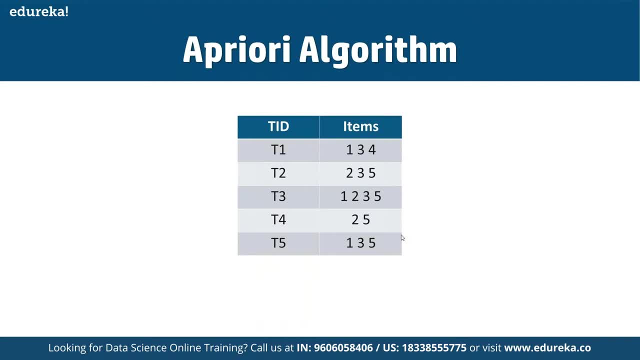 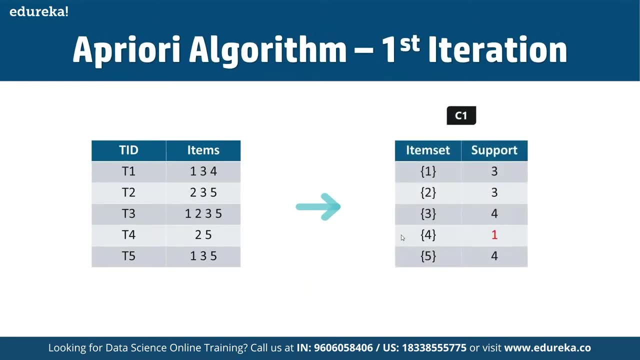 three five, one two three five, two five and one three five. So if you talk about the first iteration now, let's assume the support value is two and then we can create the item sets of the size one and calculate their support values as against here. 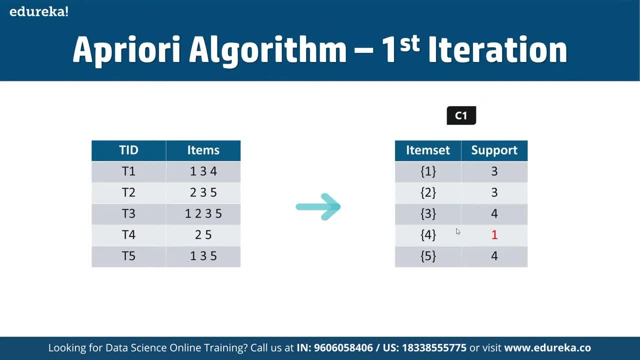 So, as you can see, of the item for has a support value of one, support value of one here, which is less than the minimum support value. So we are going to discuss For in the upcoming iterations and we have the and that's how we can have. 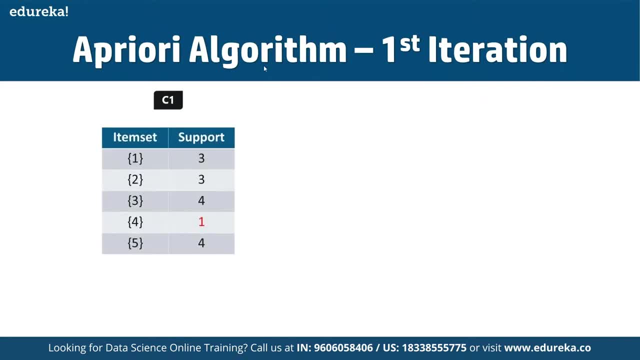 the final table defined here as the FN. So here we are going to discard the value as for, and then we are going to have the final value to be giving given to us. So the item set your support value less than minimum support value, That is, two, are going to be eliminated. 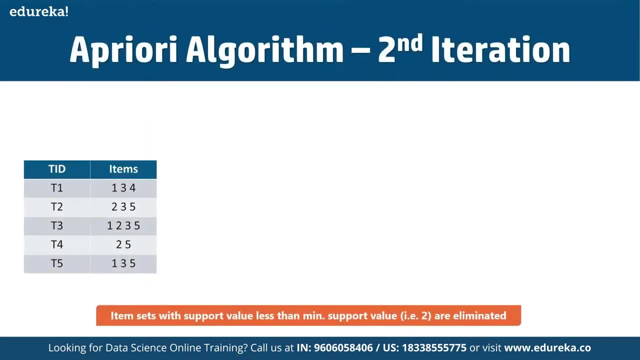 Next we are going to create the item sets of size two and calculate their support values. So all the combination of item sets in F1 are used in the iteration here. So here we have C2 and then we have the F1 here. So basically, here we are going to make use all the entire tradition here. 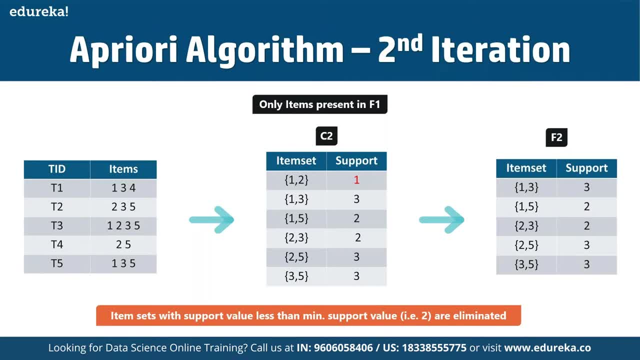 and item sets having support less than two are eliminated again, And in this case we have one and two right. So let's now understand what exactly we mean by printing and how it makes a Priory one of the best algorithms for finding the frequent item sets. 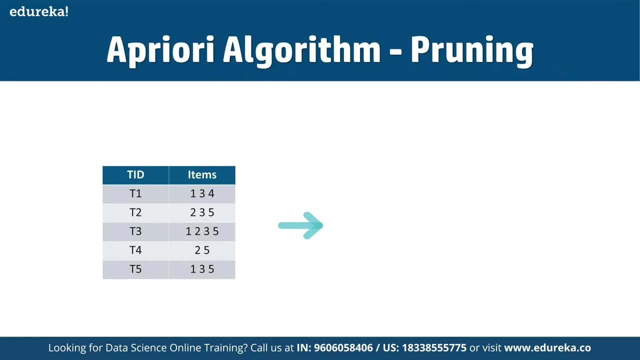 So if you talk about pruning, then we are going to divide the item sets in C3 into subsets and eliminate the subsets that are having a support value less than two from this given item sets here. So here we are going to work on the third iteration. 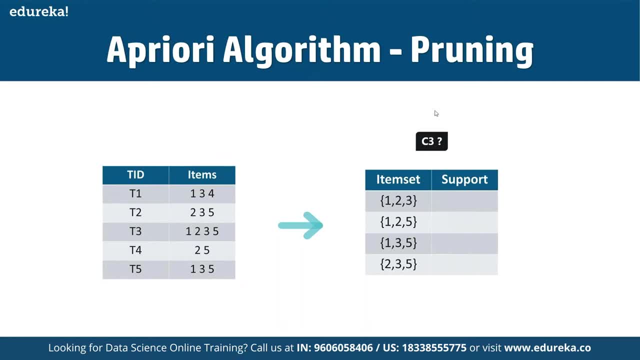 So we will discard one, two and three. We are going to discard one, two and three, and one, two and five as well. So they both, as they both contain one or two, and this means again, and this is the main highlight of the Apriori algorithm. 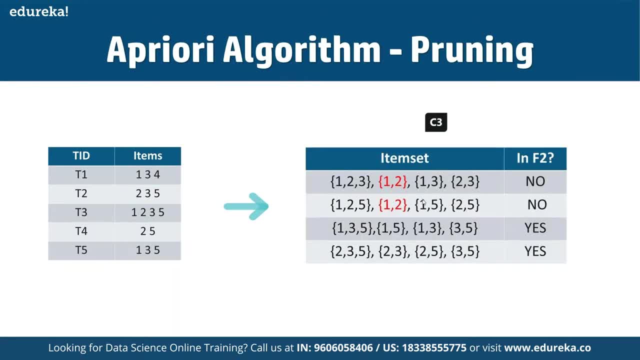 So you can see over here going to discard one and two And this is the main highlight of this entire algorithm here because, again, the one and two is a common thing available in these: both data sets right. So this is the main highlight of Apriori algorithm here. 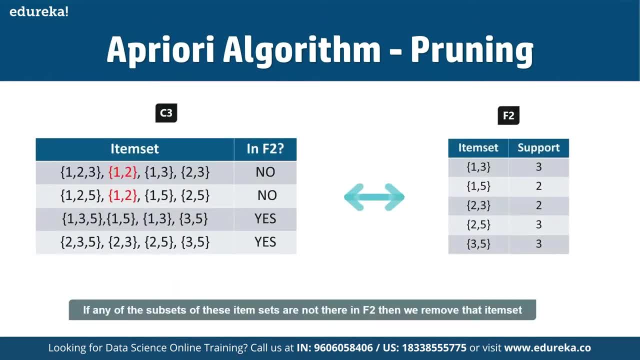 And then if you talk about the fourth iteration, so if now, as you can see, if any of the subsets of these items are that are not in F2, then we are going to remove that particular item sets. And then, in terms of the fourth iteration, 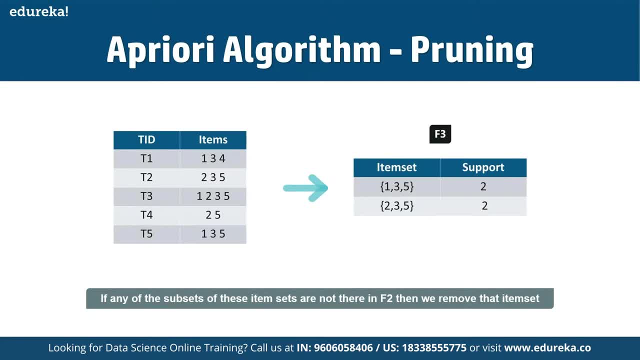 let's suppose here we have the transition ID and here we have the item set and support available. So, since the support of this item set is going to be less than two, so we will stop here and the final item sets will have is the F3 one. 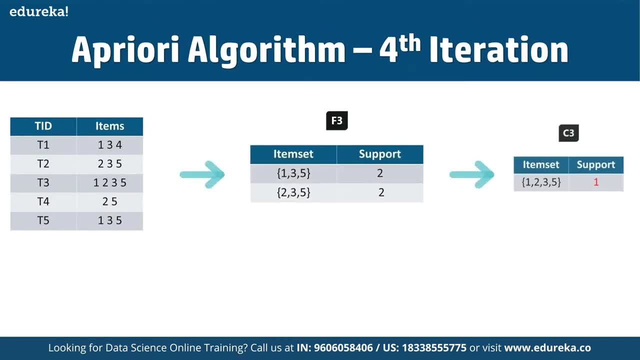 And now, still now, we have not calculated The confidence value yet. So again, this is something that we have to keep in mind. So with F3 we get the following item sets: That means for one we have one, three and five, and subsets are one, three, one, five, three, five, one, three and five. 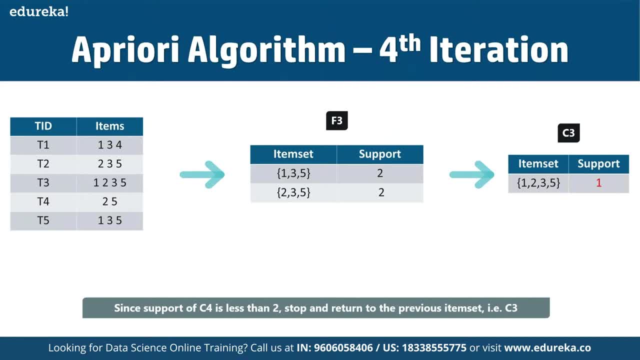 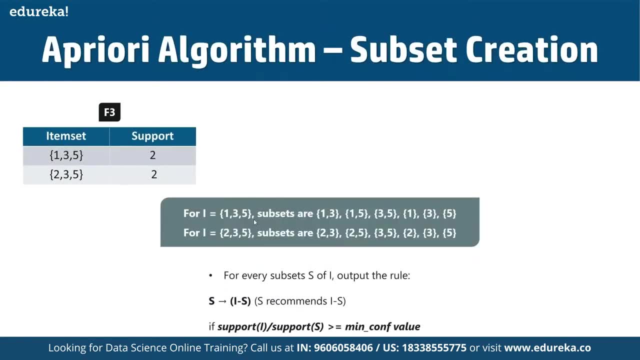 Whereas for item sets, one again we have two, three, two, five, three, five, two, three and five itself for the other diamond size available. So for one we have one, three, five. These are subsets of one, three, one, five, three, five, one, three and five. we, as two, three, five are subsets. 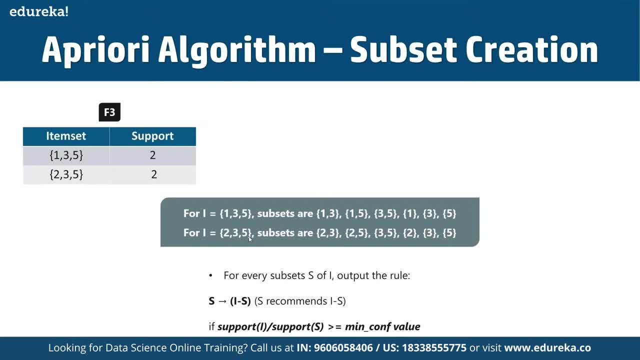 of two, three, three, five, two, five, two, three and five right and for every subset of I. we have to find the output rule Now, when we are going for applying rules here, so we will create the rules and apply them on item set F3.. 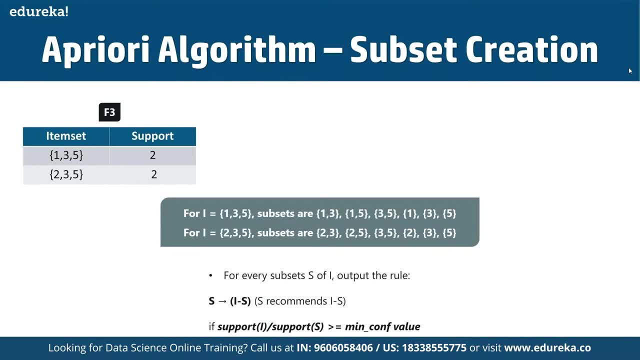 So now, let's assume a minimum confidence value is 60%, so for every subset of whether that we have S of I, so are, the output rule is going to be: S is going to be Recommended, so S is going to simply recommend is, and then we hit support, it is I, and then we can simply divide this. 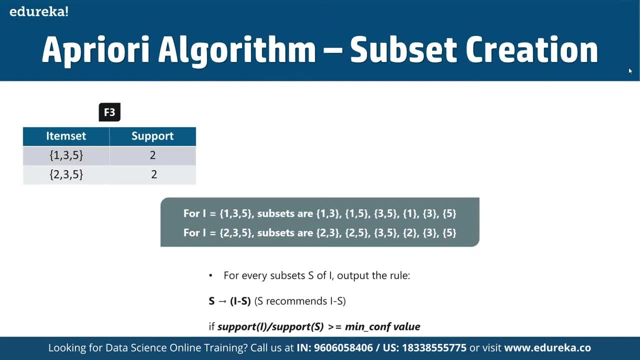 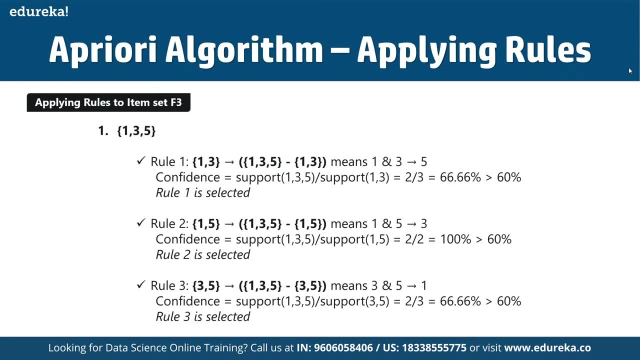 by the support cell And to find the minimum confidence value is going to be one to five. So your rule one here is one, three is again a subset. means that means one and three will result to five. That means if a user is purchasing one and three, both the items, then 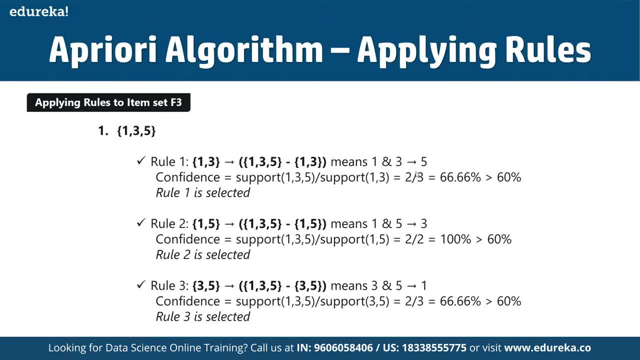 we have a good possibility of the customer going for the fifth item as well. So here the confidence is going to be: support one three. five divided by a support one three, that is two by two, that is 66.6%, is 60%. so here rule one is going to be selected and in rule two 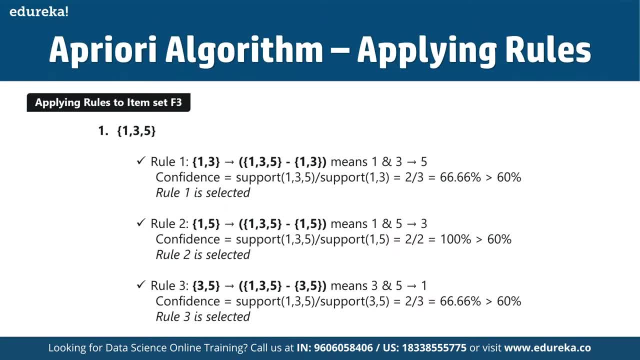 We have one five, one three five minus one five. That means if the people, if someone is purchasing one and five, then they are going to have a good possibility of going for three as well, where we are going to see the confidence and support for finding the confidence. 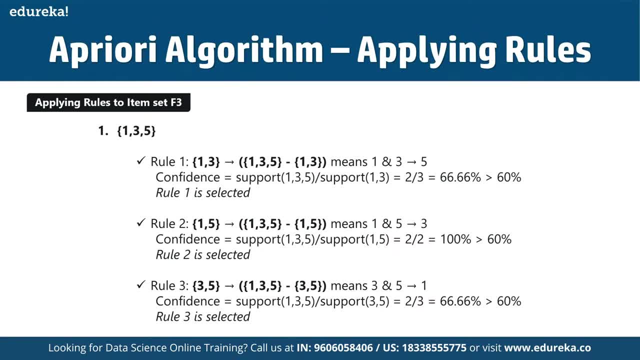 We are simply going to again subtract support for one, three, five by support of one, five, There's two by two, and this is going to simply be translated at 100%, and which is much greater than 60% as well. and same way in rule three. 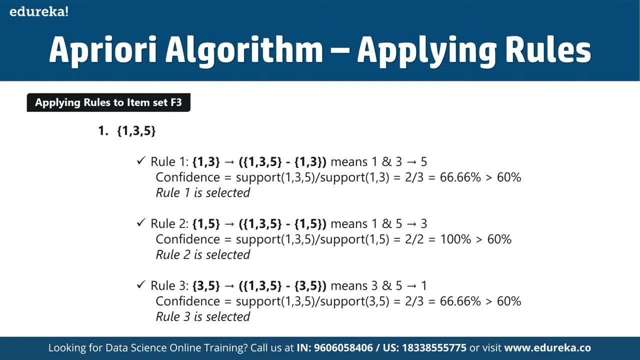 We have three, five, one, three, five, three point five. That means here if someone is going for purchasing three and five, then they are, then they are going to high possibility of going for one as well. So here the conference is Four, one, three, five, divided by support: three, five that we get. 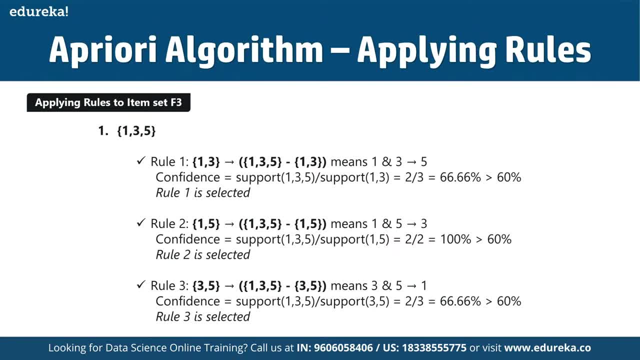 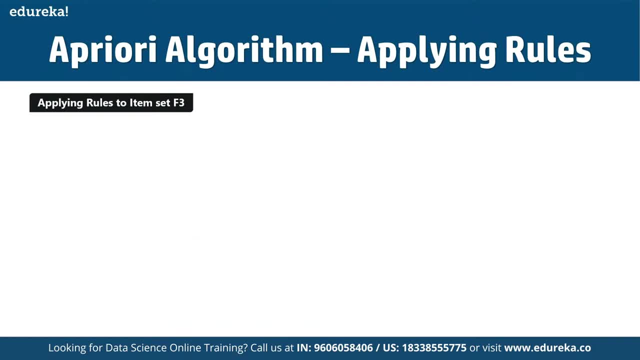 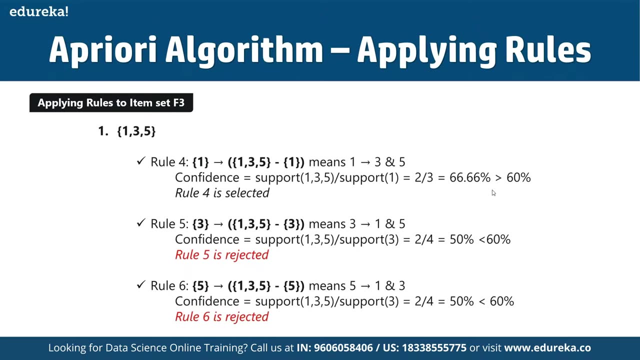 as 66.6%, and here the rule three is going to be selected here, as you can see here, Now, upright now, if you talk about the application of rules here, now, when we are talking about this rule here we can see, whenever the confidence is going to be more than six, more than 60% to find 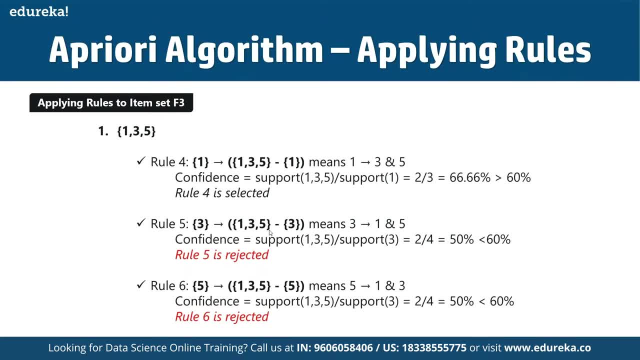 him, then this rule is going to be selected as against here, in this rule, five where what? where those who are purchasing three, they have a possibility of going for one, five, both. So here the confidence is less than 60%, which is why this is going. 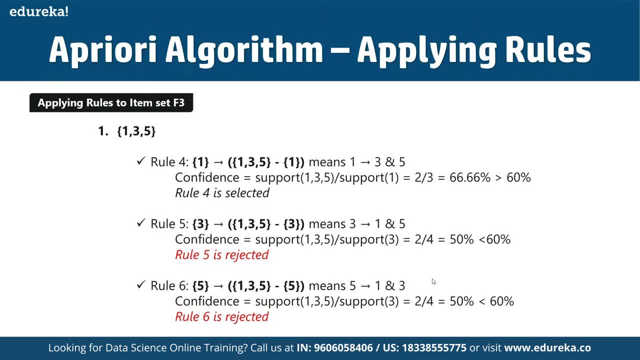 to be rejected. same way for rule six as well. Same here for rule six as well. because here the confidence is going to be less than 60%. then that's why this is going to be rejected here. Okay, because again we have, we have assumed a minimum confidence. 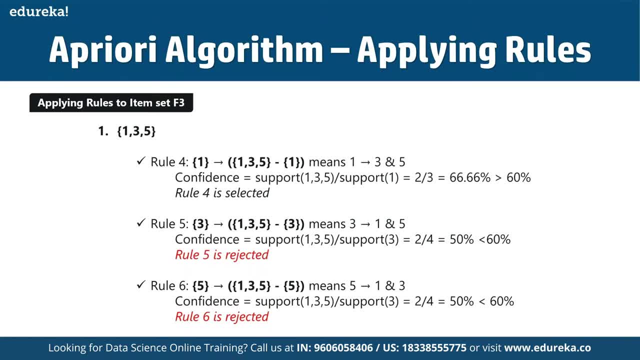 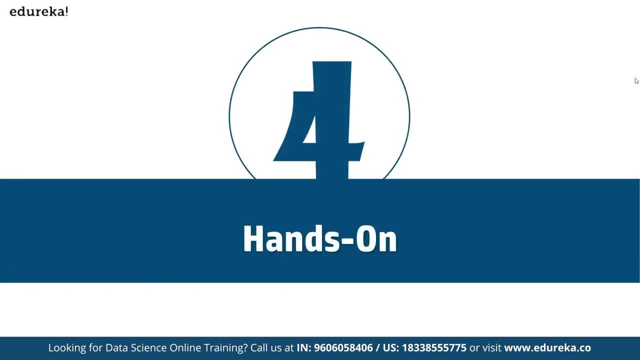 level for 60%, and wherever we are going to get the confidence less than 60%, We're simply going to Reject that particular model here. All right. So first of all, that's how we have seen how we can create rules in a proprietary algorithms here. 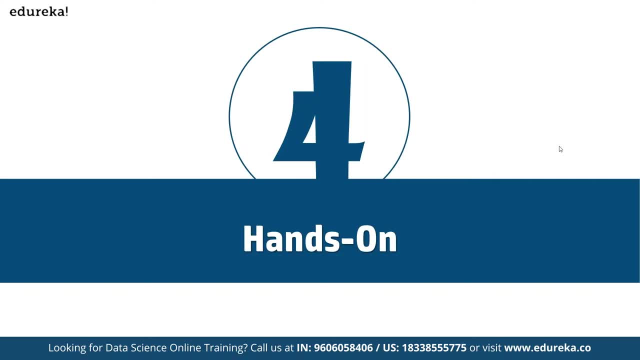 And the same steps can be implemented for this item: set two, three, five, and then we are going to try it and see which rules are accepted and which rules are going to be rejected, and how we can implement the a priori algorithm in python. All right, 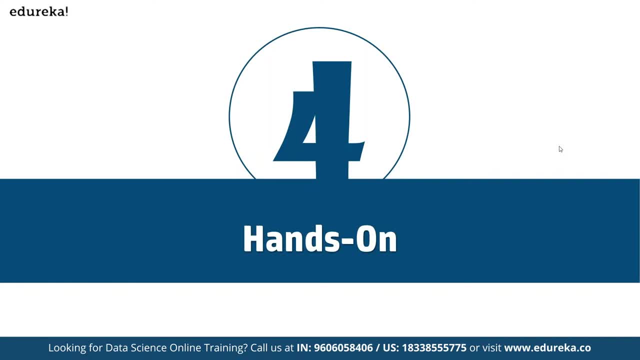 So let's fetch some sample data sets here that we are going to work on. So to get started working on the actual analysis here. We are going to make use of the pie charm ID, so we can use any of the ID, or we can also make use of the python hormone, ideally. 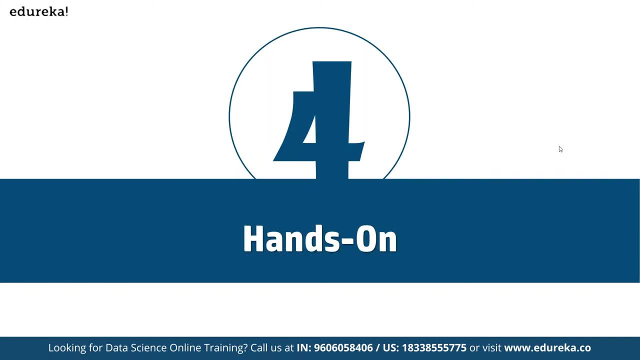 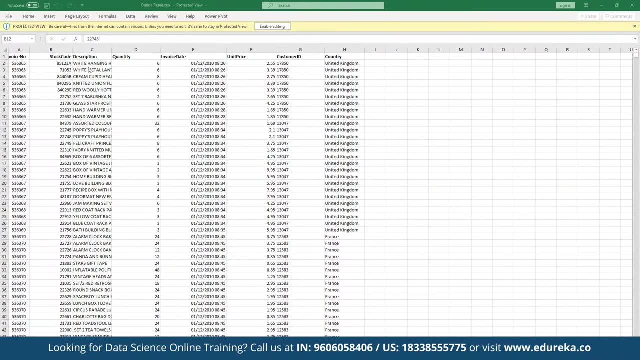 to get started. So we are going to make use of pie charm In this file- will be having the access to the invoice number. We have the stock code, We have description, quantity, Invoice date, unit price, customer ID and then we have the country. 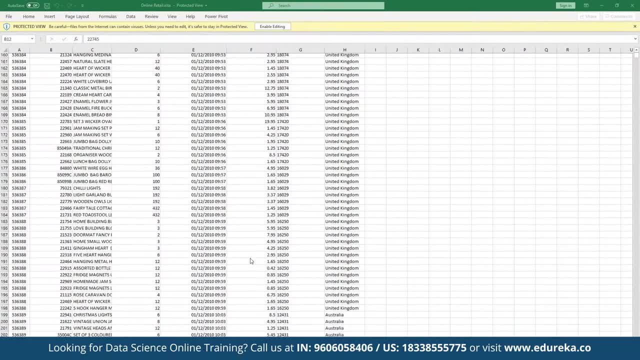 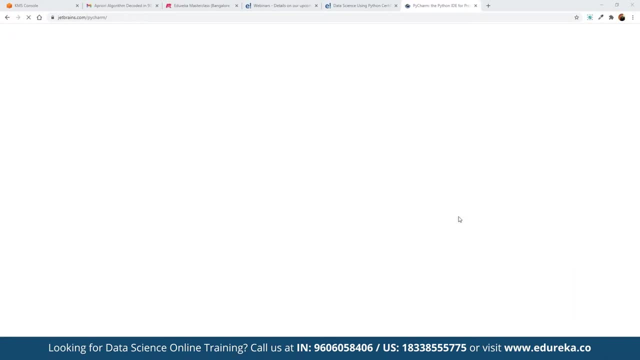 So this is a data point, that this is a file that we are going to work on, All right. So in the meantime, we are also going to install pie charm as a main ID. So in case you want to work on python and we can make use, 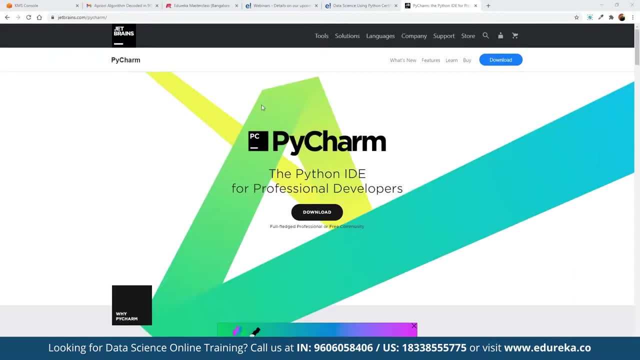 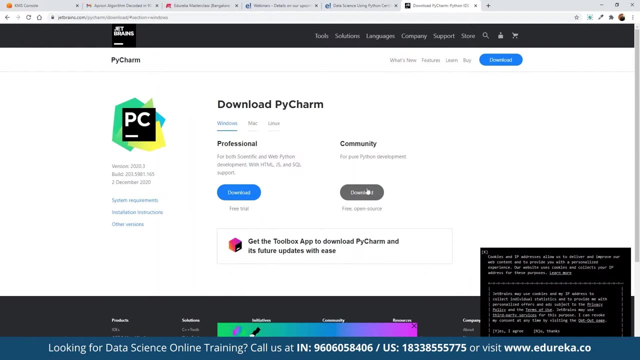 of pie charm ID, which is one of the most popular IDs for getting started, and pie charm is also offered as a free tool. That means here we get is also offered as a community tool here, So you can use it as a community tool. 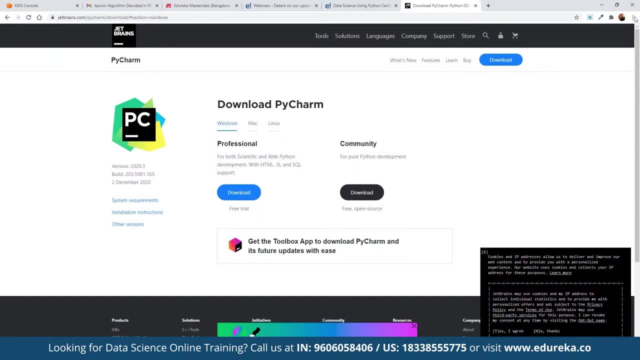 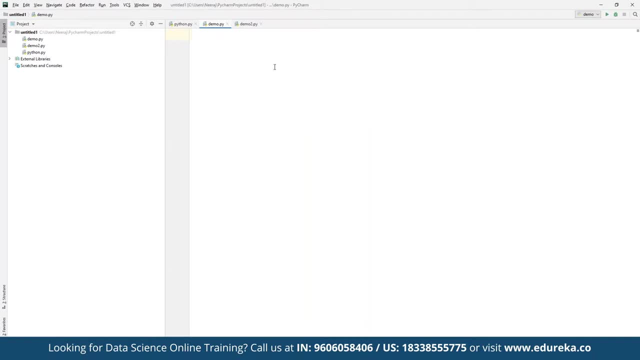 In order to get started. So once we have the access to it, we can open this up. All right, So here we can get started first. First of all, we are going to work on the pandas library. So here we are going to import pandas and mlxten libraries imported. 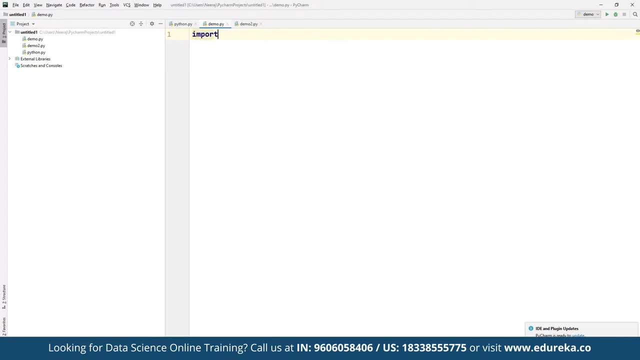 and to import and read the data set. So here we go, going to choose import and then here we are going to find import pandas And from pandas as PD. So here we go to import pandas as PD And then we are going to use from mlxten. 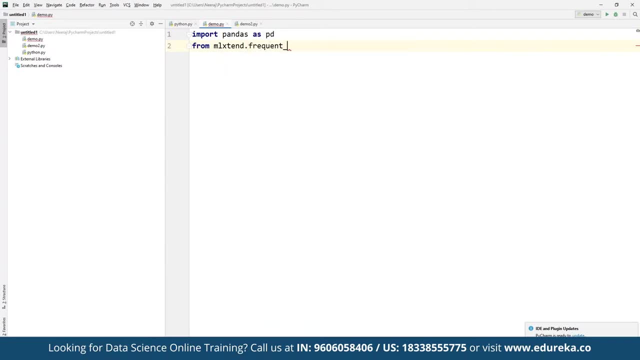 We are going for frequent dot frequent patterns. We are going to import a priori And then we are going to use the same from mlxten dot frequent underscore patterns. We are again going to import association rules. They're going to pull. We import Association rules and then we are going to create. 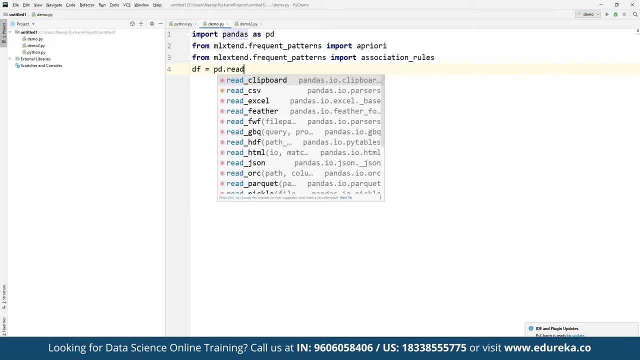 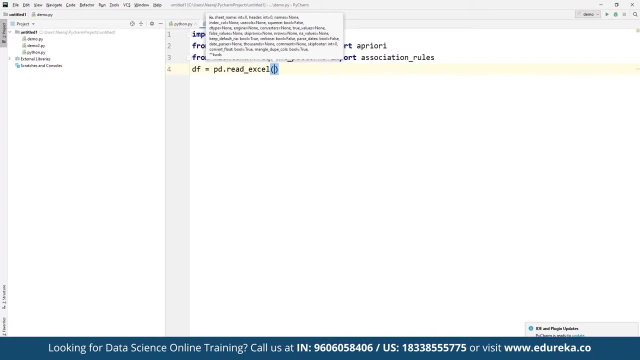 a data frame where we are going to make use of pandas diary as PD dot read, and here we are going to read Excel file. If it if it is a CSV file, let me define it as read CSV and here we can define the path, suppose here. 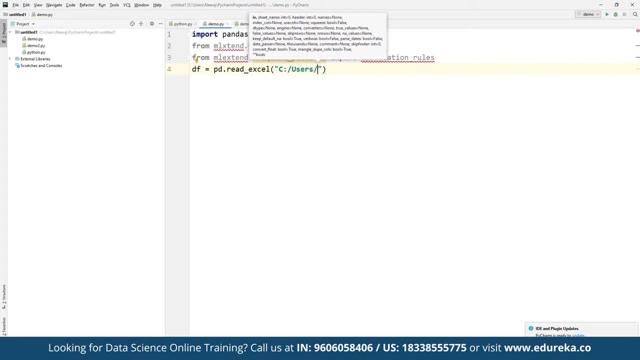 The file is currently available in our users location and the users we have it in downloads and by the name of online underscore retail Excel is six. So this is the three that we have currently imported here And, in case suppose, some libraries are currently missing here. 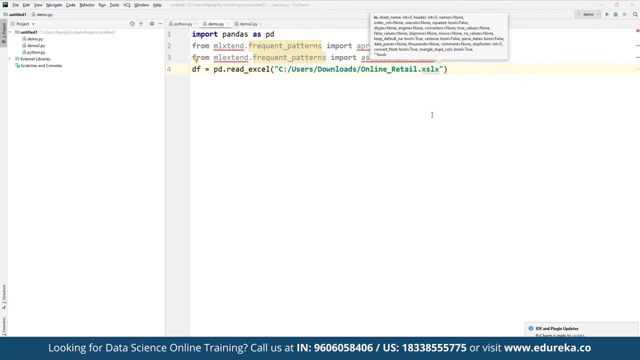 So we can import these libraries as and when required here. Suppose, if we, if something is missing here, we can simply import these libraries in case they are not properly installed. So for installation of any new library here we can go to file under settings here. 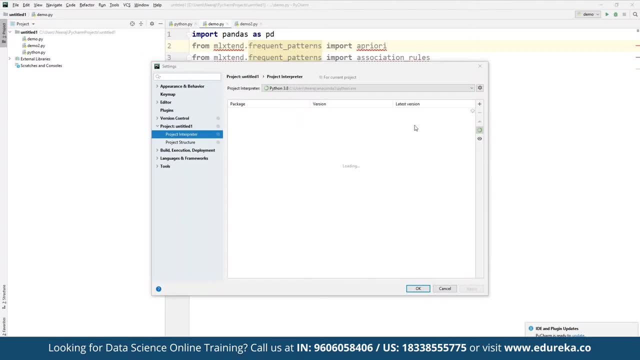 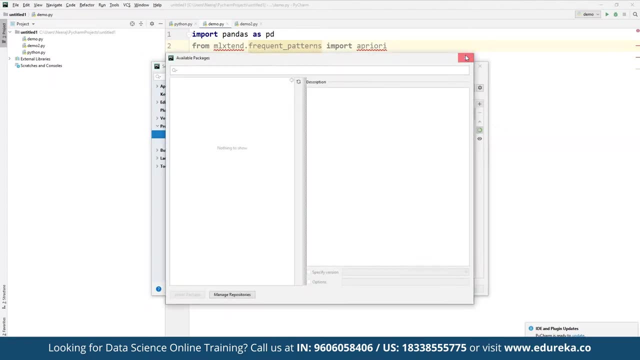 We have to go to Project interpreter. in case you want to add any specific library here, then we can simply click on plus and then we can choose which all library we want to add. here We can simply see the entire list of all the libraries currently. 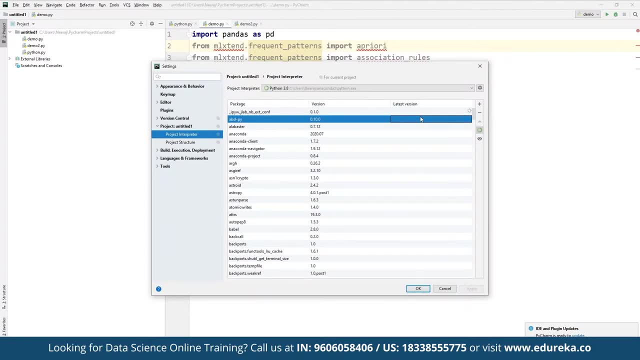 installed here And now. if you want to start with more than we can simply add more libraries, and then we can start deploying it one by one. So for example, suppose, if you want to install any specific library here, so here we can say: let's say, here we want to install the. 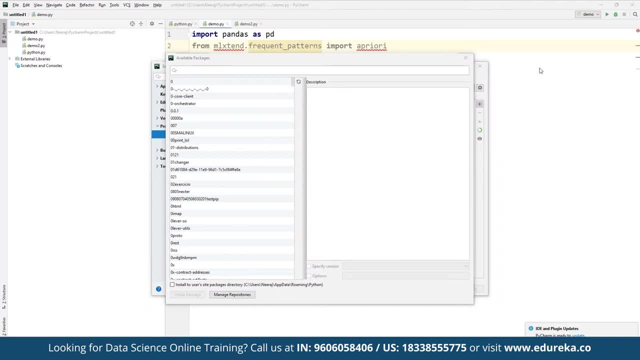 a priori here. So if we can see how we here, we can also import the MSN. So if this library is currently available, we can simply click on install package and this is going to be installed and stored in a system as a library. same way, if you are looking for a priori. 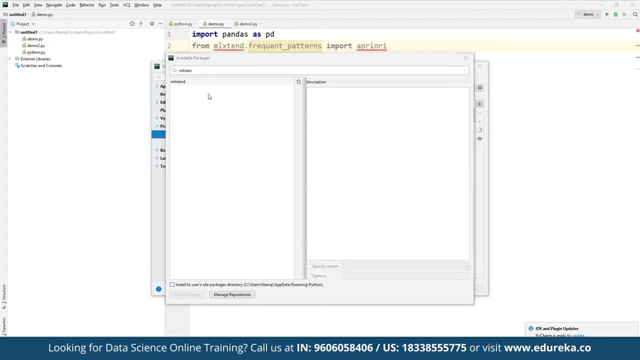 here. So here we can also use, because again, at the end we are going to use a priori from the MSN that we have imported. So here we are going to install the other package as well. So the first package for a medicine has been installed, and now we 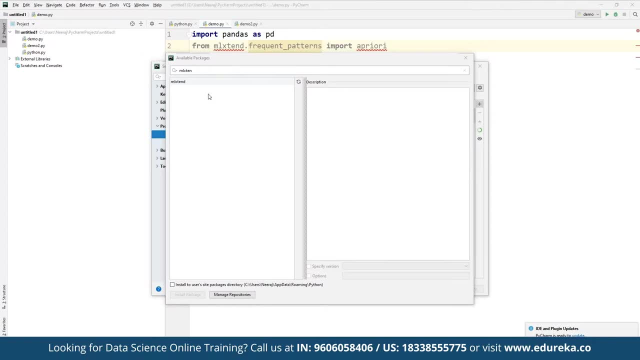 are, and if you want to install the other packages, then we can also install it. So in case we have missing some kind of library, that we can simply install it, or in case we are, we have not used those libraries out and we can simply use them one by one. 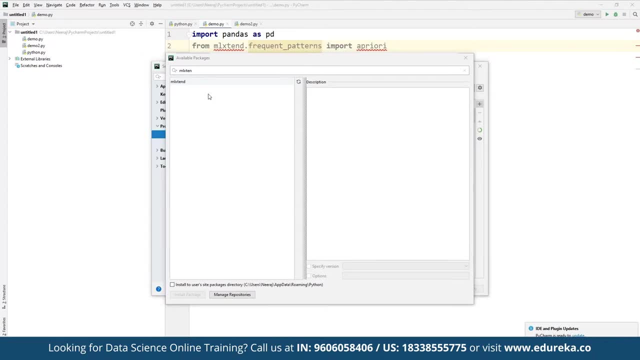 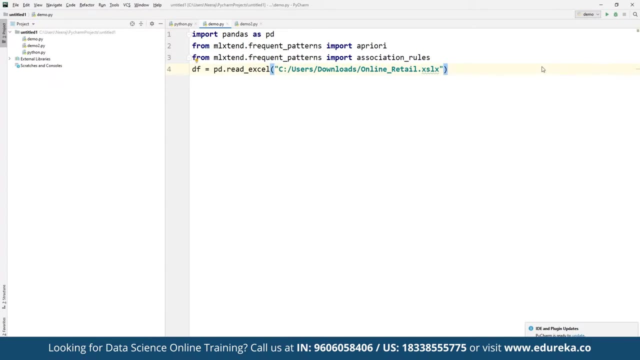 So, once we are done, we can simply come out. So, as you can see now, once the libraries have been properly installed and we will be able to see there is no error being shown here, And this is the path of the file: that where we have stored online. 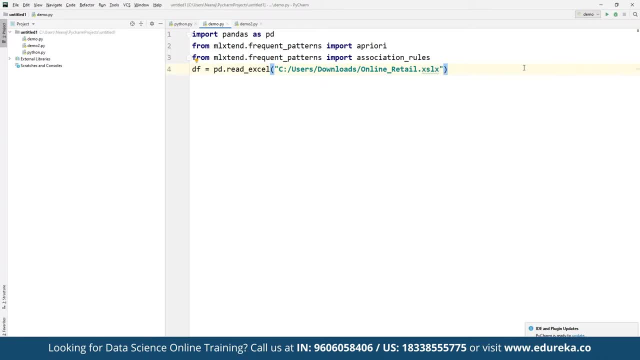 retails dot xls file here. So just to confirm, we can confirm that we do have the file by the name of online retail dot xlsx available here in a download directory. So once we have specified the file here and then we are going to simply use data frame dot head. 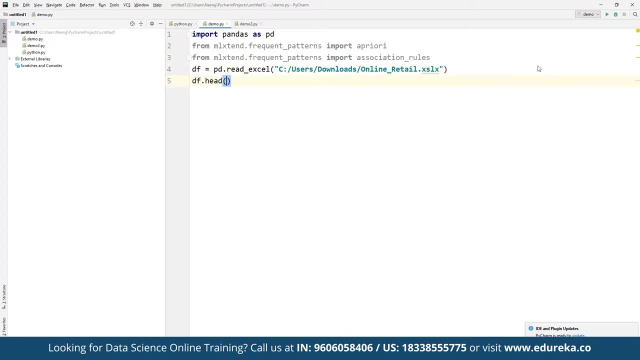 So in case we want to see the first few entries of the current data set that we have imported, So here we can simply define DF dot head and then, from the given path, the first two head are is going to be returned back As a response. 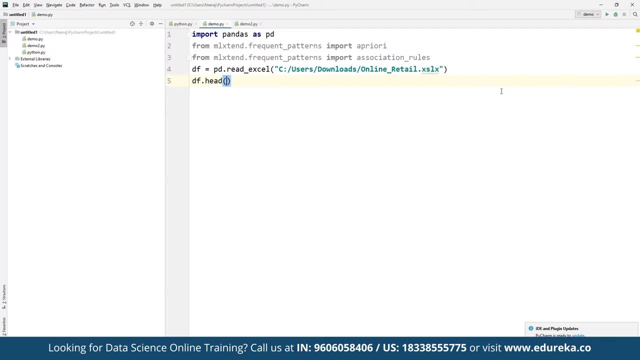 Now, once we are done, we can simply start applying it Now, once we have the access to the data set here. next step is going to be focus on data cleaning, which will include removing spaces from some of the descriptions that we have, and for that we are. 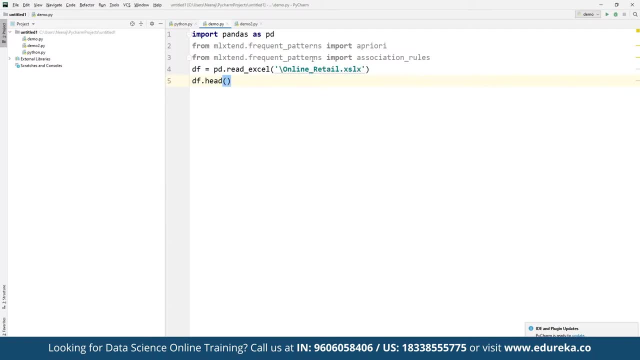 simply going to specify here We get now, instead of using the data page, the data frame head here. So now we are going to use the data frame and then from here we are going to add a short description. So here we can add a short description here. 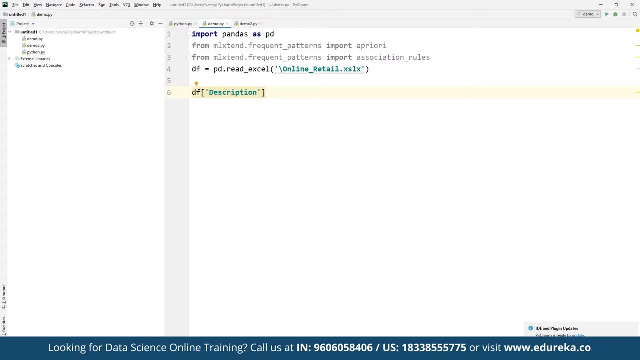 So, basically, we are going to do work on data cleanup, which includes removing spaces from some of the descriptions, and then we are going to drop the rows that don't have invoice numbers and remove the credit transition as well. For example, suppose we have some rows where we don't have the where. 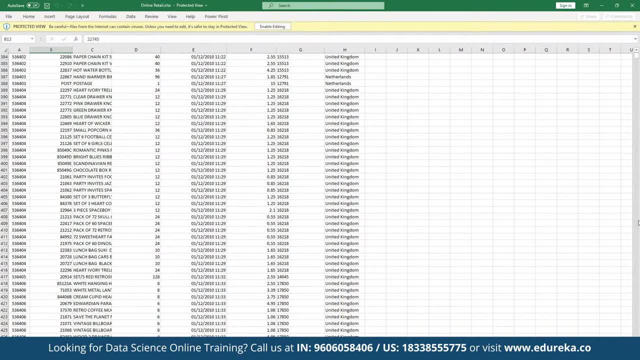 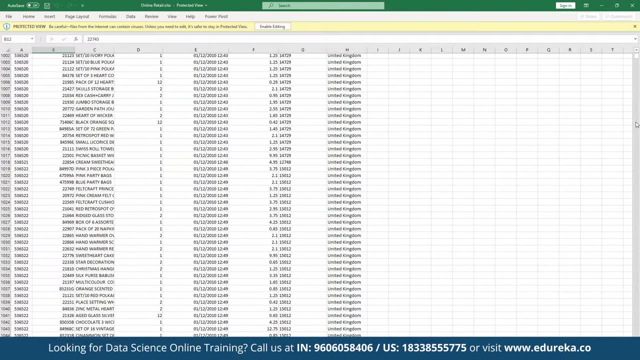 we have blank Transitions, itself right. We have some blank invoices and then we have invoices numbers and remove the credit transition where we don't have any kind of invoice number. All right, so we have. we are going to be here. We have to work on removing those kind of anomalies. 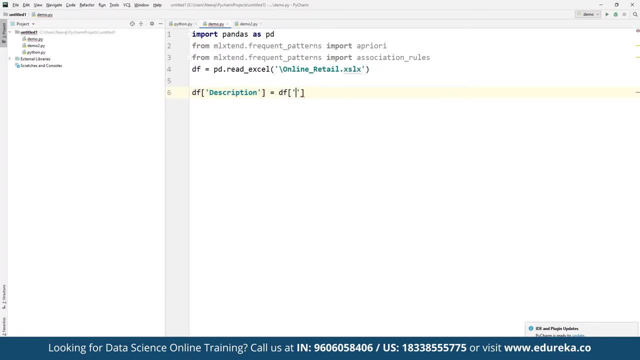 So you have from the data frame. So here we can add parameter as description. Now on a description, we are going to use a string function as string dot strip. So stream functions available under string. We're going to make use of it. 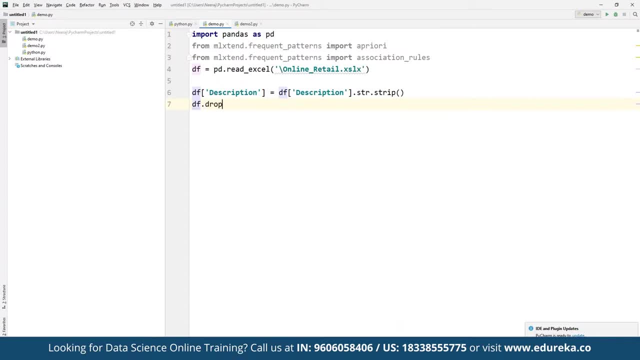 And then same way from data frame We are going to work on dropping. There we can find the values for X is equal to 0, and then the subset where the. what kind of values we have to drop? Do you have to define that parameter? where the invoice number? 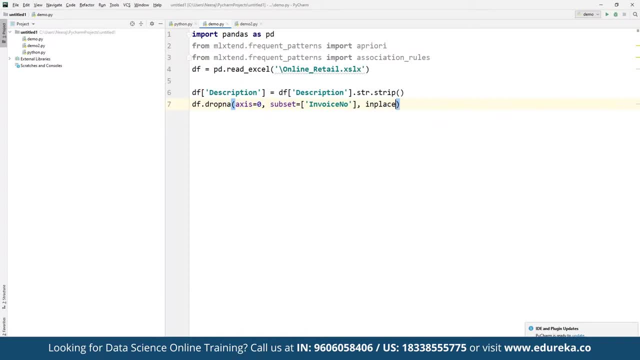 Is going to be in place is going to be true, And then from data frame we can define the invoice frame, Invoice number And then we can define it to be our data frame. We're in voice number again. We are going to convert that to a string itself. 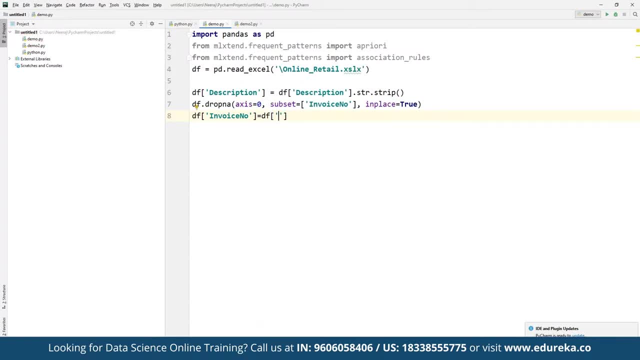 We have, we can define data frame and then the invoice number type. So here we have invoice number Dot, the AS type, and then we are going to the SD type here. But again here we can keep it to AS type. So here we can define to be a string value. 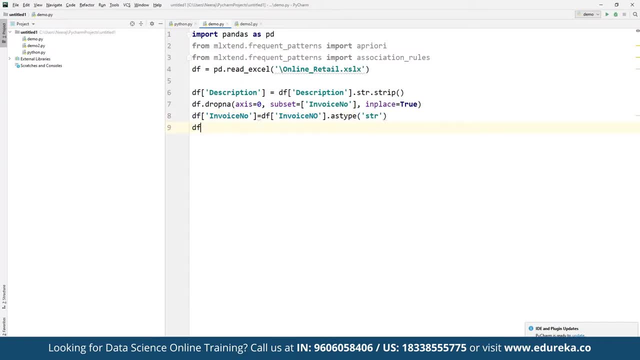 So here we can find to be a string and then we can create a Data frame where we can find data frame should be a value closer, Okay, the value closer to data frame where we are going to find the invoice number. So here we have invoice number and then we can define this as a string. 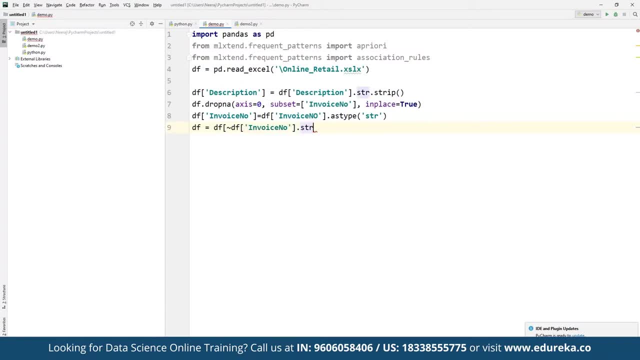 Point missed on the. so here we are: string dot contains, and then we can define wherever the value is C, wherever the value is C as a part of definition defined Here, and then we are going to simply save it as a part of given data frame. 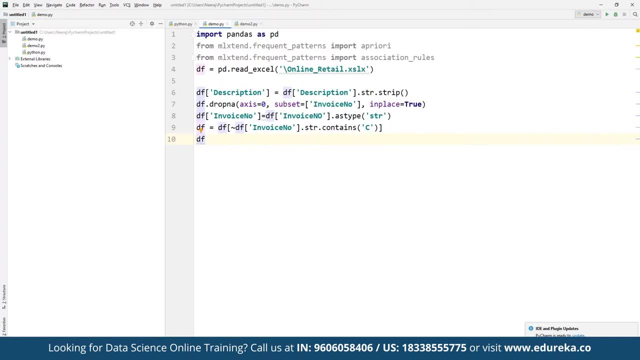 So after we are done cleaning up, we need to consolidate the items into one transaction per row with each product. So for the sake of keeping the data small, we are only going to look, we are only going to be looking at a sales for the for any specific country. 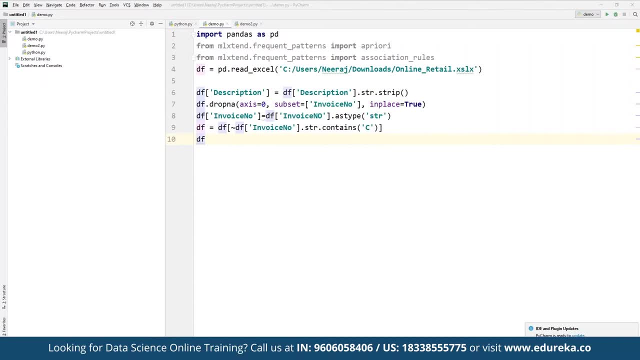 So now, once we are done, we are going to create and consolidate the items into one transactions per row with each product and, for the sake Of keeping the data set small, we are going to look at the sales for a specific country. So for that, let's say here, we want to focus on one country data set here. 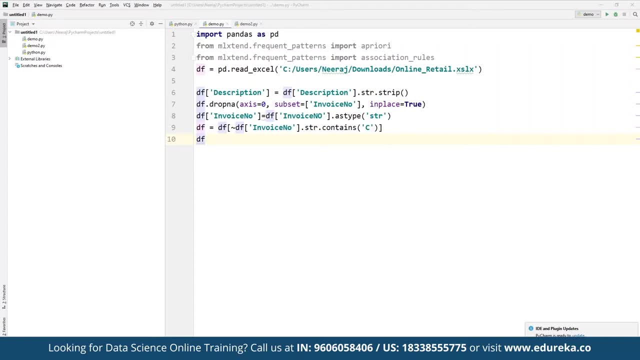 So here we can use basket and then in the basket part, here we can define multiple data frames. For example, first of all we can define data frame and here we are going to use the same data frame and then we are going to segregate it further based on the country itself. 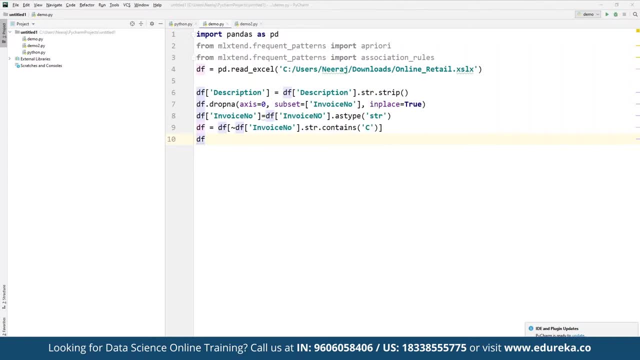 So here we can find country and then under country we can define which country we want to focus On. the country should be suppose, let's say, France, as a single country. So here we can define France as a country that we want to use for consolidation, and then we are going to group. 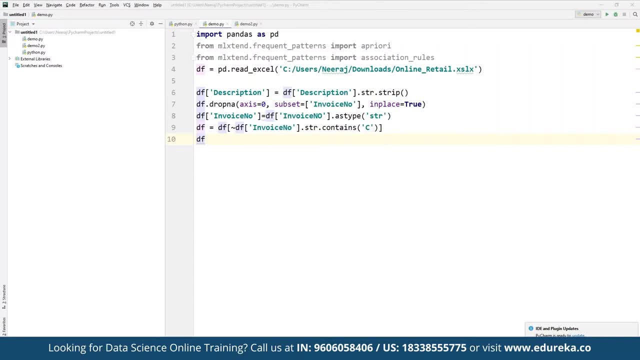 So here we can use group by the invoice number. So here we are going to find the invoice number for it. So here we have invoice number, And then we can add a short description here. So here we can add Description, And then, after we are done defining the description here, we can then define the quantity here. 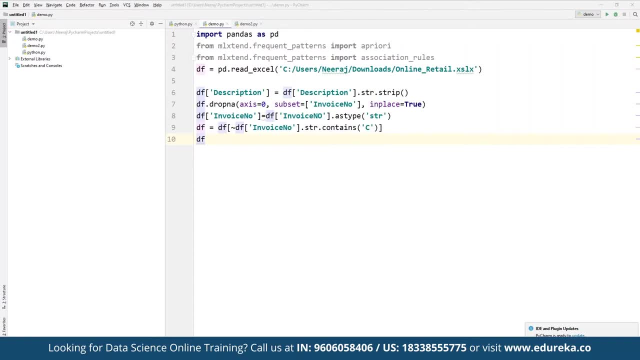 So here we can define quantity, and then after quantity we can define some. Let's put this underline. just to what the confusion? So here we can define some, And then we can define unstack Dot reset. We missed one of the time. 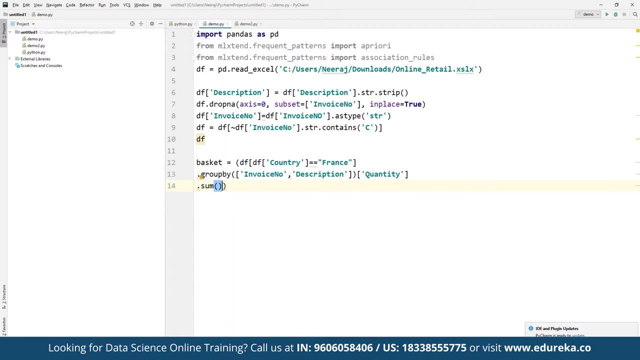 This is just so, here we get to help you to define some. and then we have defined unstack, and then we have to find dot reset, dot reset, and then the index value, here with the final any, with the final Okay, so the simple fill, color with the simple fill, and then we can find it, the value to be a simple zero. 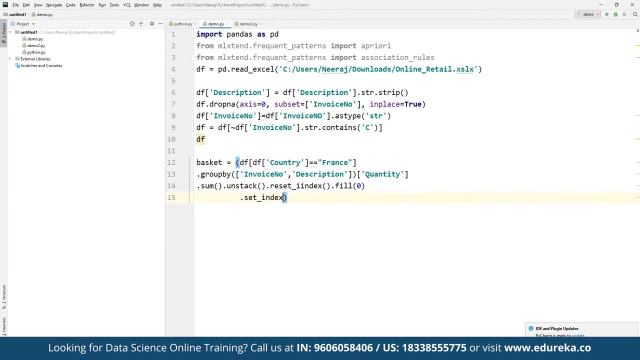 And then we can use set underscore index Where we can define for the invoice number. So here we have invoice number defined And then we can define this for a basket. So basically, here we are going to define The consolidation for the items into one transaction per row with each particular product. 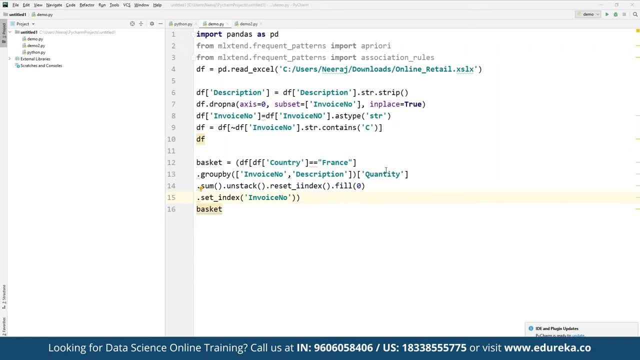 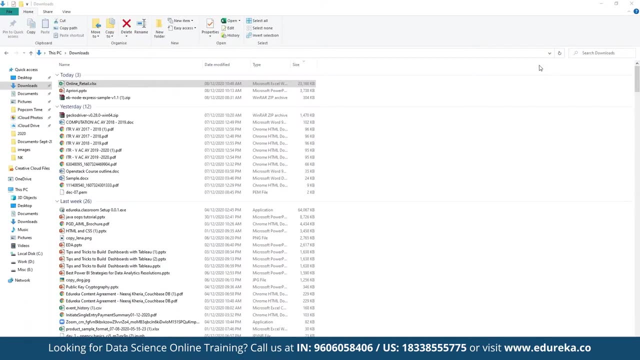 And the key, the number of transition. do we have? Yes, Focus our attention only for a for single country. It's as in France. So afterwards, so after we are done with that part, next we have to work on removing all the zeros. So basically, there are a lot of zeros in the data. 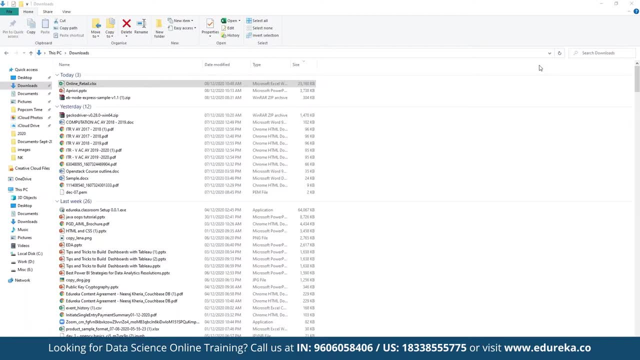 but we also need to make sure that any positive values are converted to a one, and anything less than zero is also set to zero. So for that we are going to make use of this. So, basically, here we are now for converting that. here We are going to make the 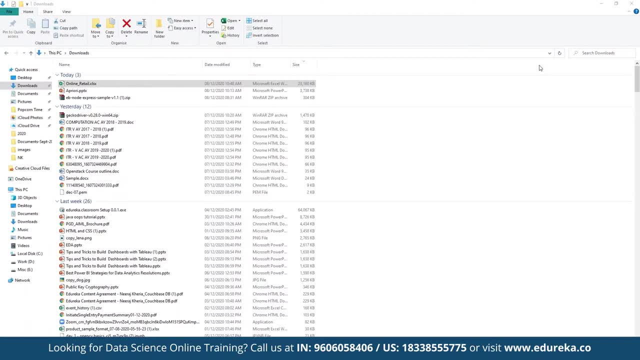 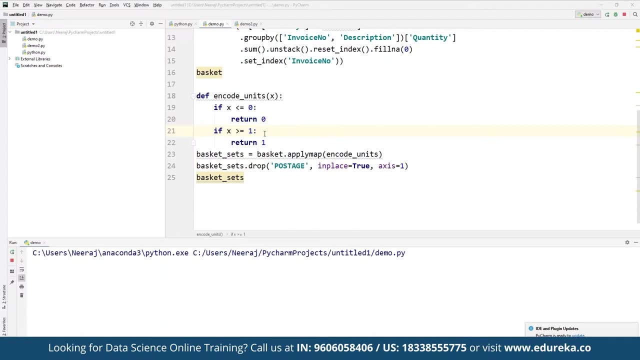 go ahead and perform the encoding SL. So here we can define encoding units. So if X is less than or equals to 0, then we are going to turn 0, and if X is greater than or equals to 1, then it is going to turn 1. 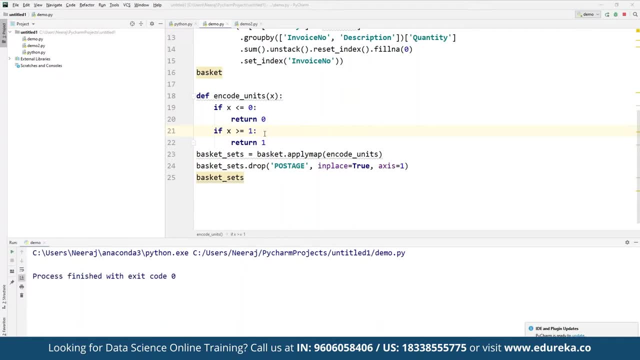 where we are going to define the basket sets and the basket apply map in code units And then we are going to use- simply use the drop postage and place set it to be true here. So basically, here we are going to simply work on, first of all, removing, removing all the anomalies here. 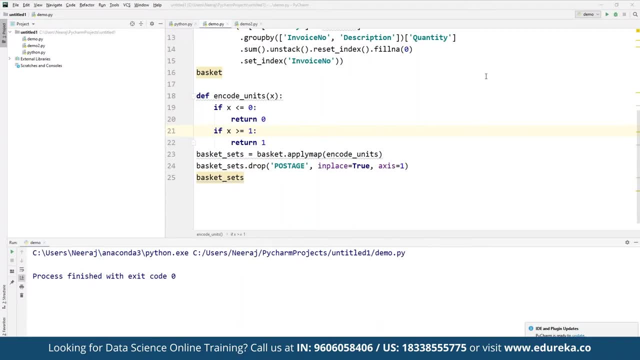 And then, if there are a lot of zeros in the data, we also have to make sure that any positive values is converted to one, and anything less than 0 is all. the sub is 0. That's what we had done here And then